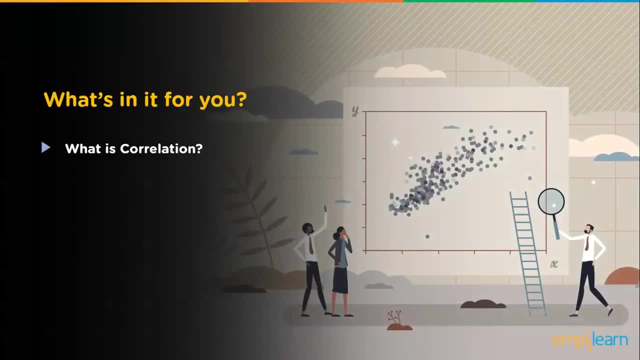 for today's session. We will start this tutorial by understanding what is correlation. Then we will move on to discuss the two types of correlation and correlation coefficient. After that we will see the limitations of correlation and some real-life applications of correlation. So let's get started. 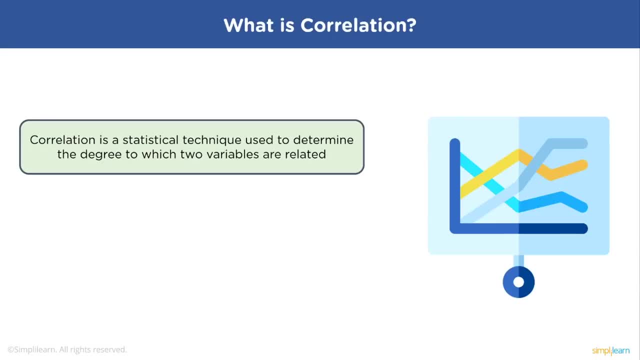 What is correlation? Correlation refers to a statistical relationship between the two entities. It measures the extent to which the two variables are linearly related. For example, the price and demand of a product is in correlation. They are linearly related. The value of correlation. 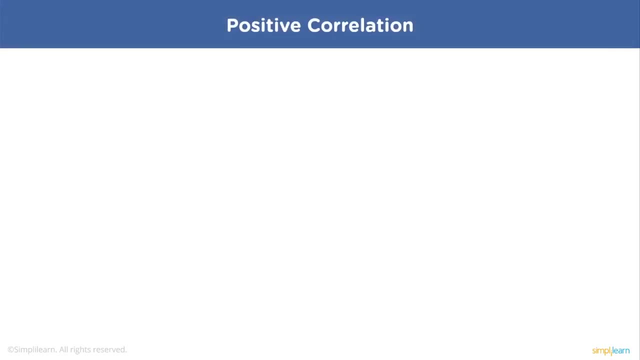 always lies between minus 1 to plus 1.. There are mainly two types of correlation. The first one is positive correlation. A positive correlation means that the linear relationship is positive and the two variables increases or decreases in the same direction. The number of trees. 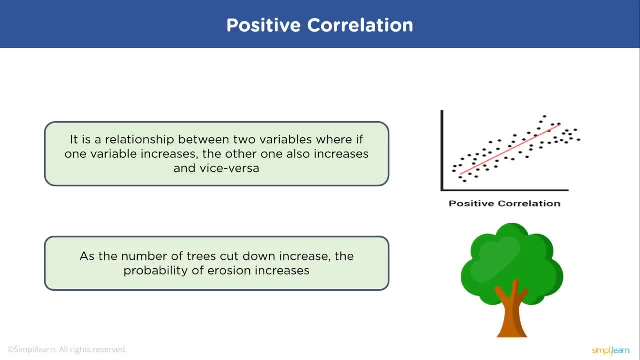 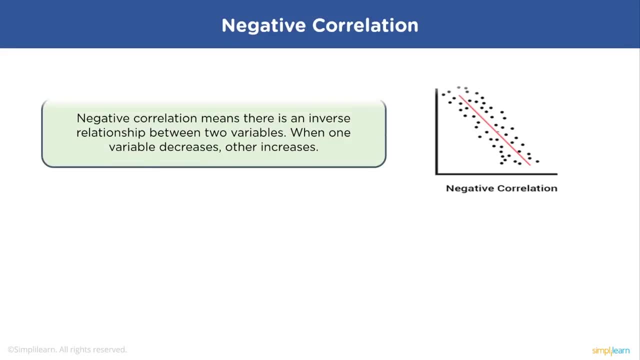 cut down and the probability of erosion are in correlation. When one increases, other also increases, and vice versa. Negative correlation: A negative correlation is just the opposite. The relationship line has a negative slope and the variables change in opposite directions. For example, if you decrease the speed of 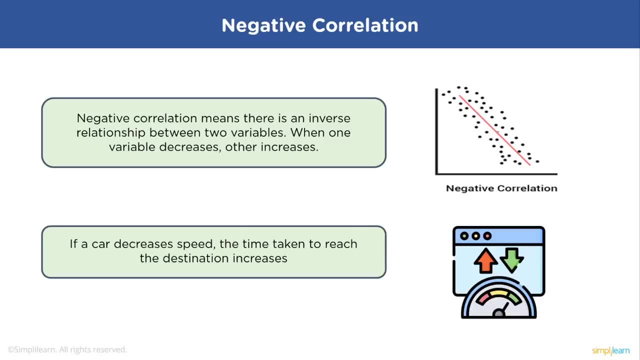 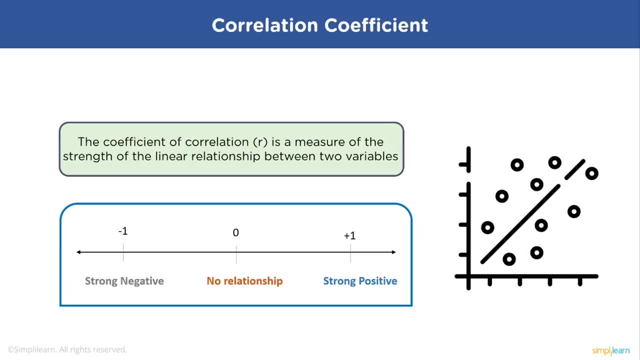 the car, the time taken to reach the destination increases. This is a negative correlation Correlation coefficient. The correlation coefficient, which is denoted by r, gives us a measure of the strength of the linear relationship between the two variables. The value is denoted by the letter r and it. 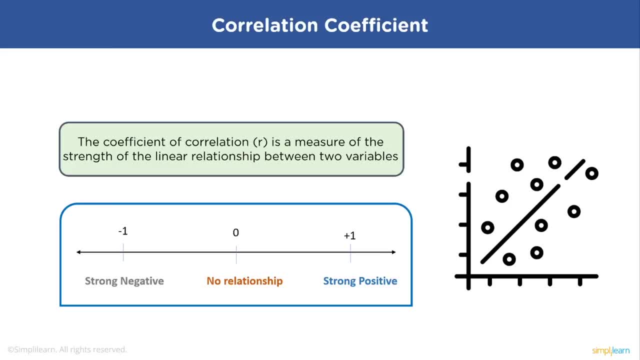 ranges from minus 1 to plus 1.. If it is less than 0, it implies that there is a negative correlation. The minus 1 indicates there is a strong negative correlation between the variables. If r is greater than 0,, it implies there is a positive correlation and plus 1. 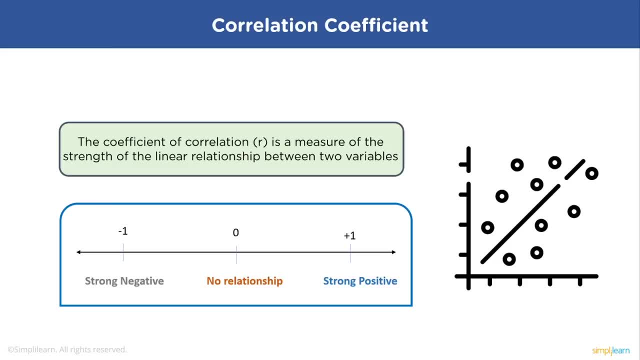 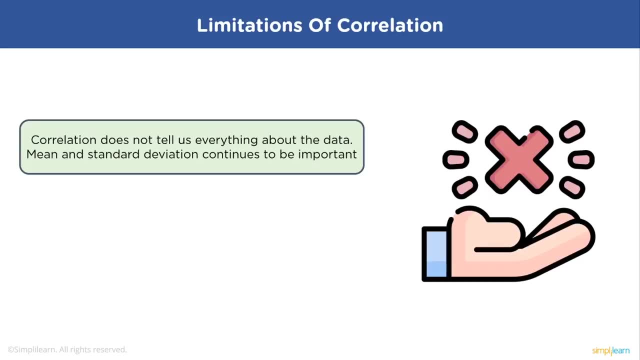 is the strongest point of a positive correlation. When r is equal to 0, we can say that there is no correlation between the two variables. There are also some limitations of correlation. The first one is: correlation does not give you every insight on the data Mean and standard.